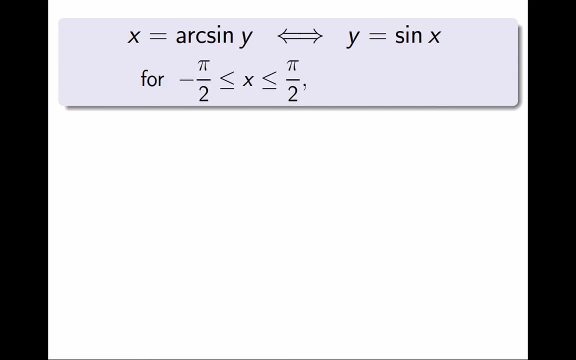 As long as x and y are in the right intervals. This is for all x between minus π over 2 and π over 2 inclusive, and for all y between minus 1 and 1 inclusive. If this went too fast, I invite you to watch the previous two videos. 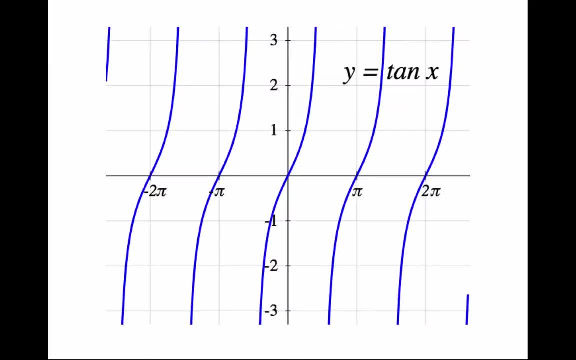 Okay, then let's try to do the same thing for tan. Here is the graph of tan. Notice that the domain is NOT all the reals. tan is not defined at any odd multiple of π over 2.. Like sin, tan is not 1 to 1, and it does not have an inverse. 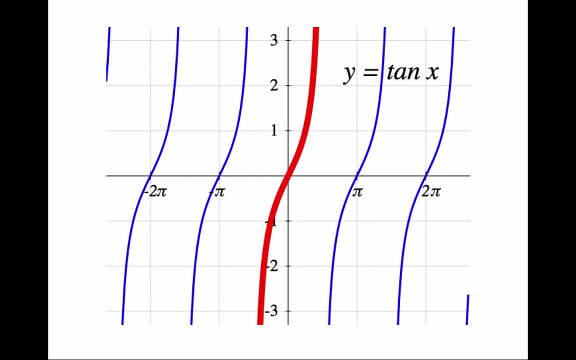 Like we did for sin, we can reduce the domain to make it 1 to 1.. It is standard to consider the function defined by just this piece of the graph in red. Then it is 1 to 1, and we call its inverse arctan. 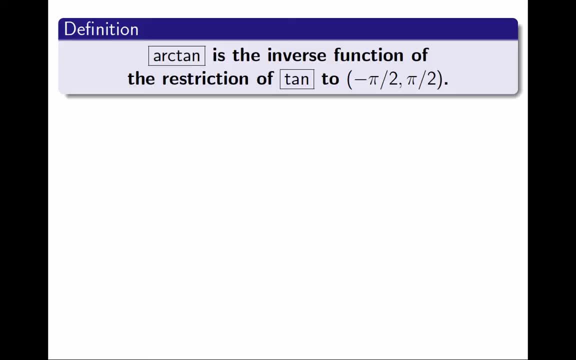 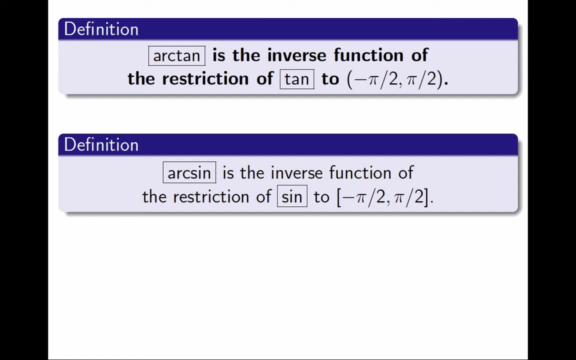 This is to say we define arctan as the inverse of the restriction of tan to the OPEN interval minus π over 2 to π over 2.. By contrast, remember that we use the CLOSE interval to define arccin. Here is the graph in blue of the restriction of tan. 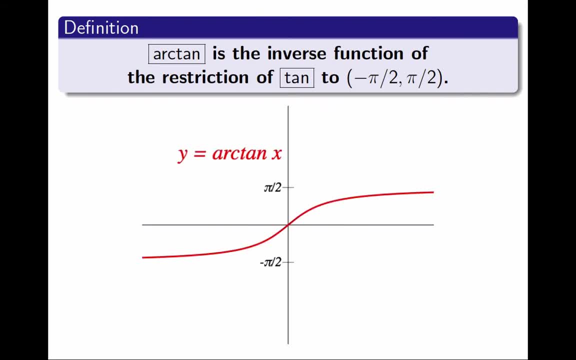 And here is the graph in red of its inverse arctan. Here is both of them together. Since they are inverses of each other, we can obtain one by reflecting the other with respect to the diagonal of the first and third quadrants. 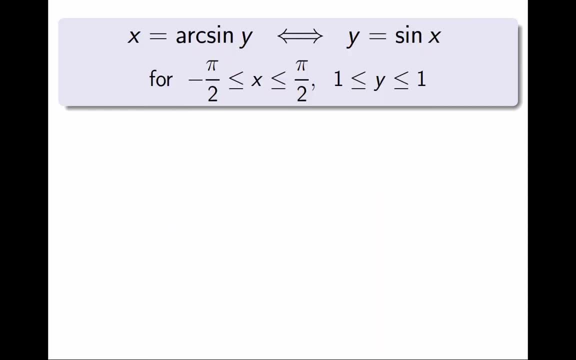 And just like we could summarize everything we needed to know about arccin by this statement, we can do the same thing for arctan. We can write that x equals arctan if, and only if, y equals tan, But this time the intervals are different. 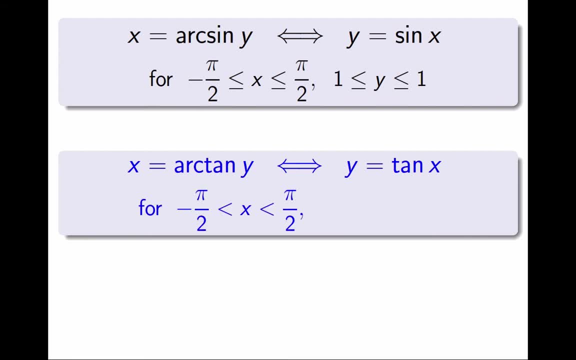 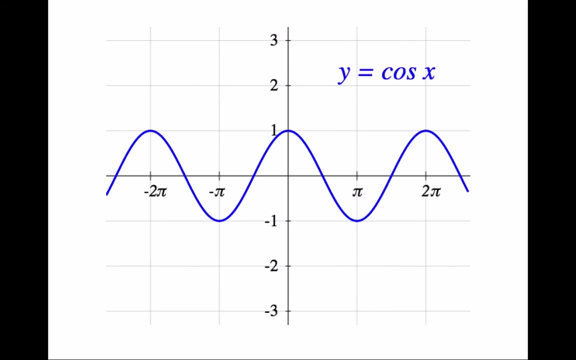 This equivalence is for all x between minus π over 2 and π over 2, not including the endpoints, and for all real numbers, y. We have one more function to go. Let's look at cosine. Here is the graph. Like the other trig functions, cosine is not 1 to 1..